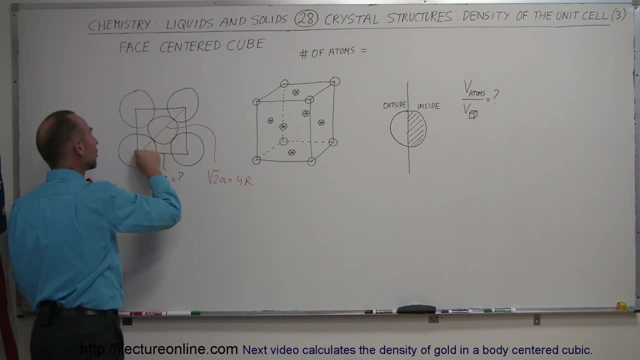 perspective depth-wise, so that the diagonal across one of the faces, which is equal to the square root of 2 times the side a, is equal to 4 times the radius of an atom. again, 4 times means 1r there, 2, 3 and 4r, So across one face. remember in the previous video we had to go diagonally. 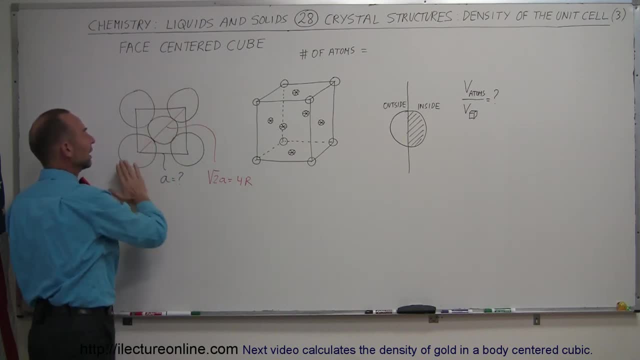 through the cube from the front corner here to the back corner on the other side. but we don't do that here. here the atoms are situated in such a way we can simply go across the diagonal of a face of the cube and therefore, in this case it's going to be the square root of 2 times a. 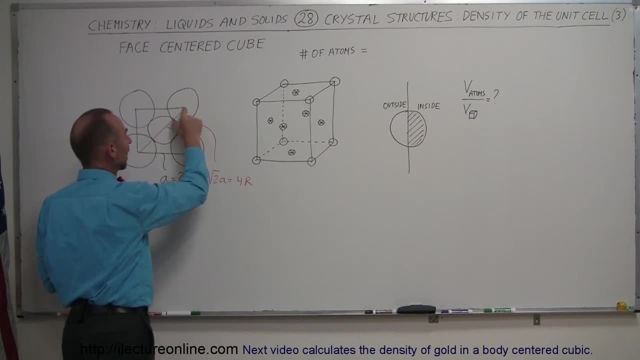 a is the side. simply, the diagonal across the side is equal to 4 times the radius 1,, 2,, 3, 4 of the atoms. So now we also have to decide how many atoms we have in one of these cubes, the way that it's packed. 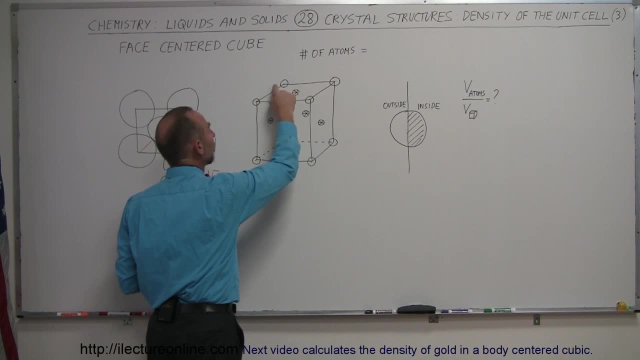 Well, we still have 1 eighth of an atom of each of the corners belonging to the cube. The other 7 eighths belong to the 7 other cubes that would be around each corner. So that would be 8 times 8 times 1 eighth of an atom belonging to the corners. 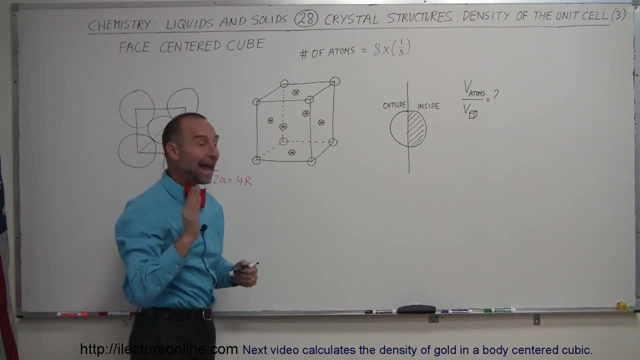 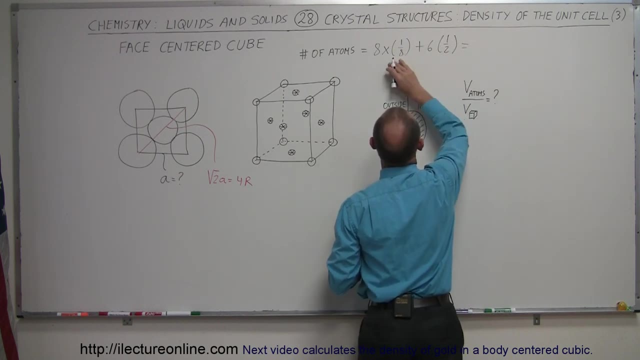 And now we have 6 atoms in each of the 6 faces and half of each atom is in the cube. So it would be plus 6 times a half an atom. So it would be 1 plus 3, which would be a total of 4 atoms, in this case would be inside the cube. 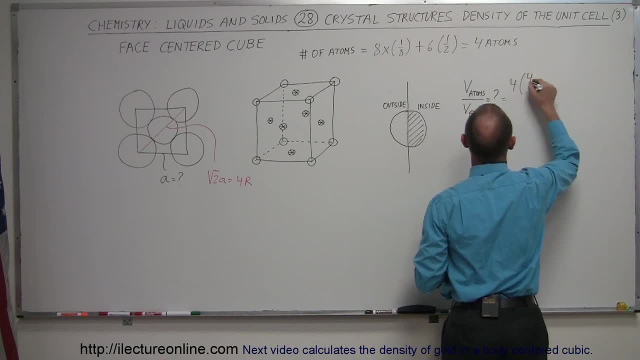 So the volume of the atoms is going to be 4 times the volume of the single sphere, which is 4 thirds pi r cubed, And we divide that by the volume of the cube, which is a cubed like that. 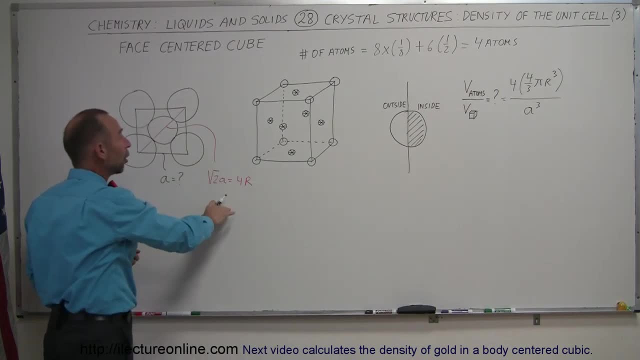 Now, of course, we have to convert from a cubed to r or from r to a. whichever way you'd like to go, Let's do it in this way. Let's solve for a and plug that in the denominator. So we have: a is equal to 4r divided by the square root of 2, and plug that in for a in the denominator. 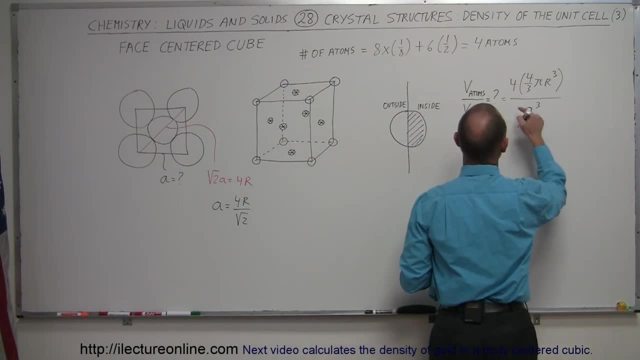 So let's try that. So this is equal to 4 times 4.. We can write 16 pi r cubed Divided by. let's take this 3 and put it in the denominator, and then we have this number right here. 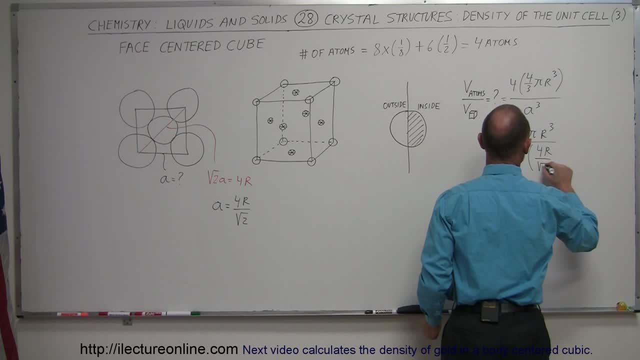 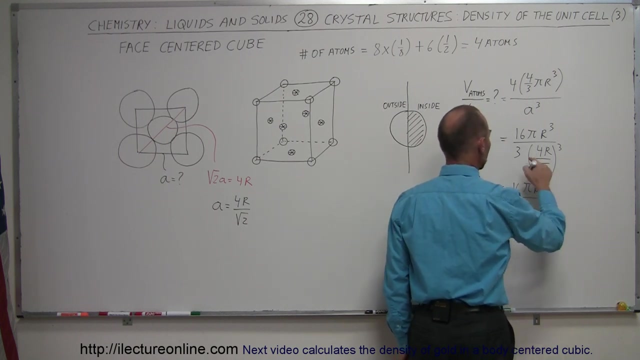 which is the quantity 4r divided by the square root of 2, quantity cubed: All right, Let's simplify that This is equal to 16 pi r cubed divided by 3 times 4 cubed is 64.. 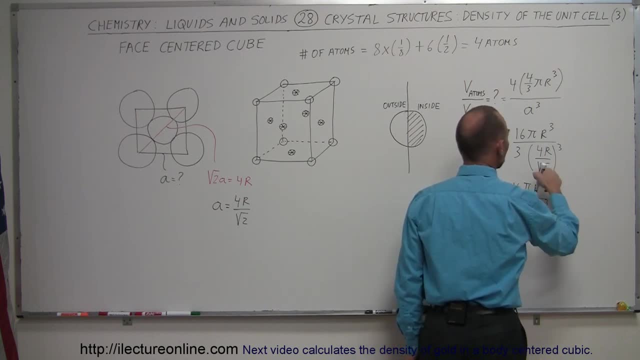 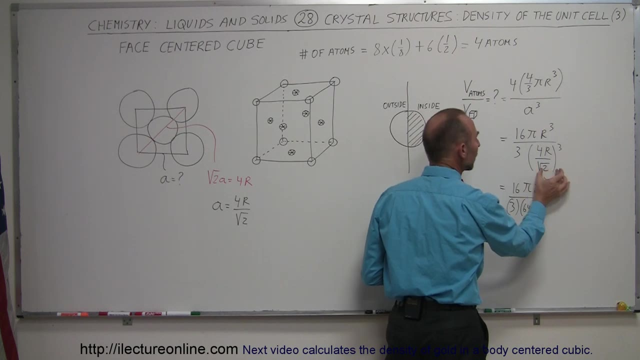 And then we have r cubed in the denominator and now we have the square root of 2 cubed. that would be 2 times the square root of 2, but since it is in the denominator of the denominator, we can move it to the numerator and write this as 2 times the square. 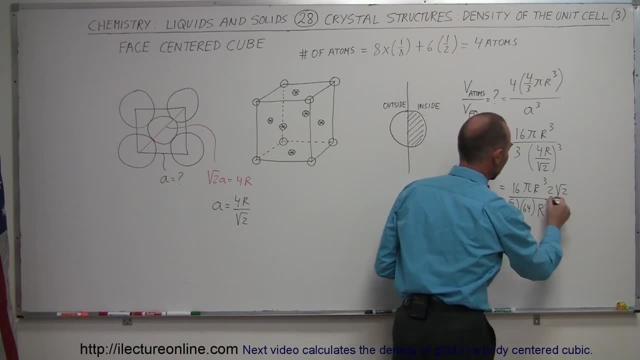 root of 2.. That is the square root of 2. quantity cubed: All right, We're getting a little closer here. We have r cubed divided by r cubed. That cancels out. We have 16 divided by 64.. 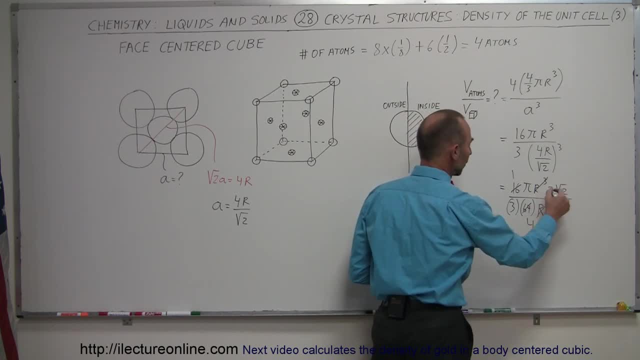 That becomes a 1.. That becomes a 4.. And we have a 2 and a 4.. That becomes a 1 and that becomes a 2.. All right, It's kind of a mess now, so let's pull out what we have left. 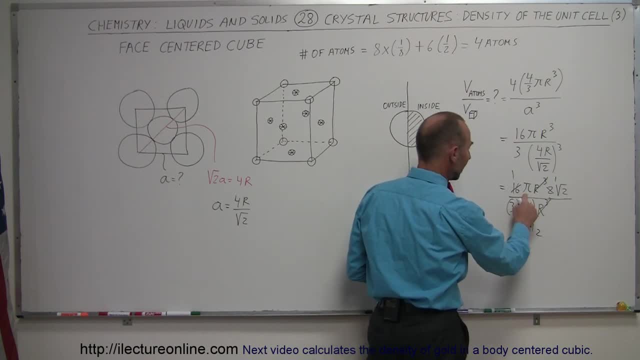 This is equal to: we still have a pi left and we still have the square root of 2 left. So it would be pi times the square root of 2.. In the denominator, we still have a 2 and a 3 left. 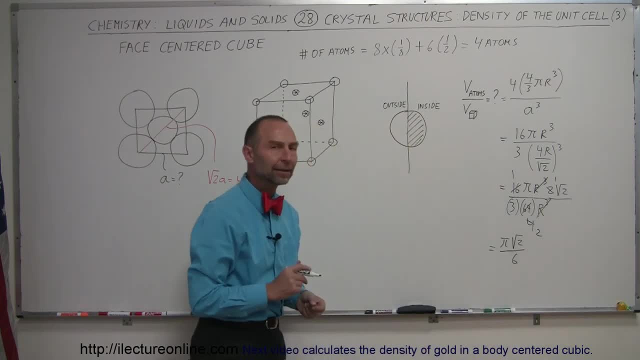 That would be 6.. So it would be the square root of 2 pi divided by 6.. I think I've got everything I needed there. Yes, Let's try that. Let's see whether that's equal to. So we have 2, take the square root of 2, times pi. 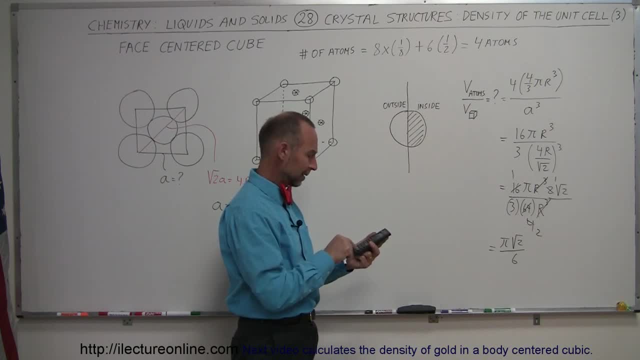 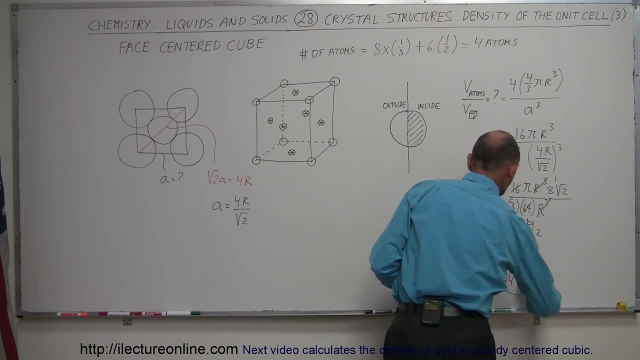 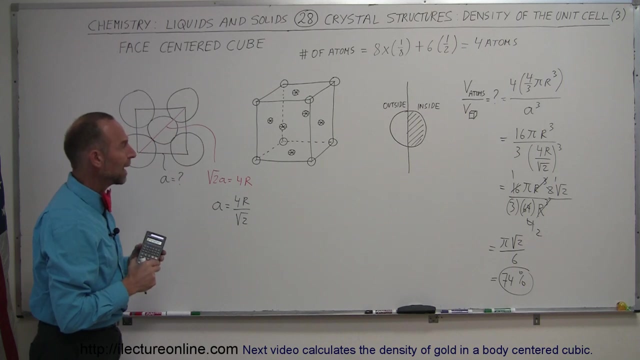 Okay, and divide that by 6, and we get 74 percent. Again, that's more than we had before, When we only had atoms at each corner. the volume density of the atoms was 52 percent. When we had a body centered, one atom completely in the middle and 8 at the corner. 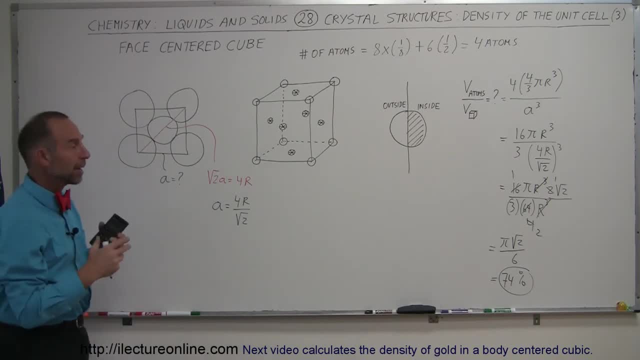 we were up to 68 percent of the volume of each cube was occupied by the atoms, But in the case of the body centered, we have a density of 74 percent. 74 percent of the space in the crystalline structure is completely occupied by atoms. 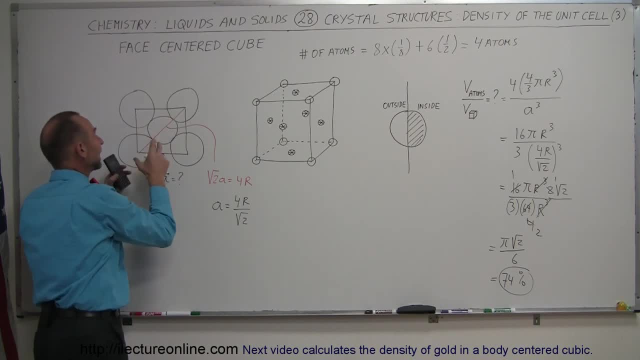 which leaves about 26 percent of little voids in between the atoms that cannot be filled, because you know the shells, the electron shells. they're pushing against each other. You can't get them any closer than that. So that's how you figure out the density of the atoms in a unit structure, for in this case, the face centered cube. 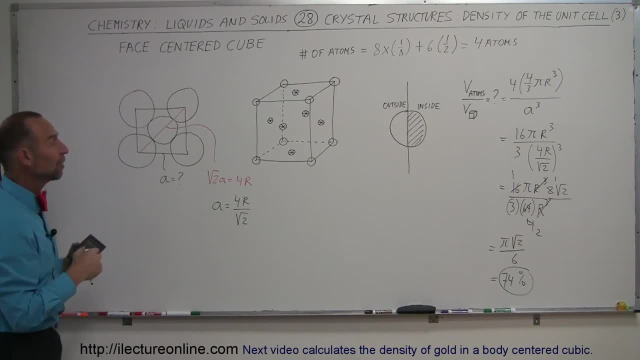 And if you want to see the other cubes, the body centered- that's a previous video- and simply the simple structure, the simple cube with only atoms at the corner. you see the video before that. So that's how you calculate the density of atoms in a crystalline structure.